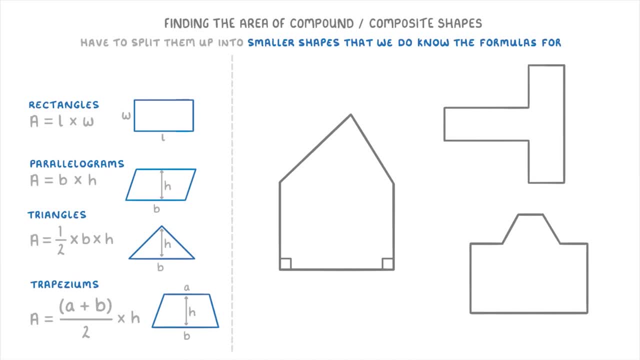 shape. the aim is to break it up into some combination of these four shapes that we know the formulas for, And one thing to point out is that we sometimes call these four easy shapes simple shapes because we have formulas for them, Whereas the more complicated shapes 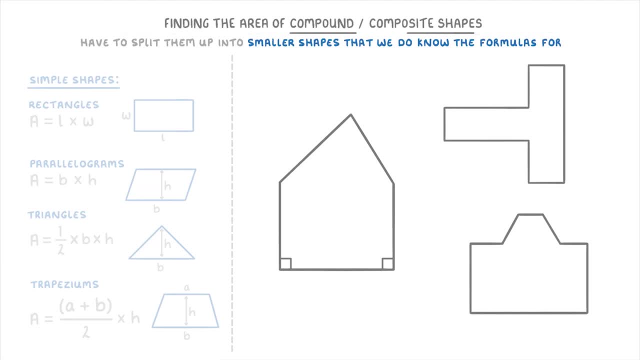 that we're focusing on in this video are often called compound or composite shapes, because they're the ones that we know the formulas for. Let's start with this one in the middle and add some measurements so that we can work through it. The first thing to spot here is that if we draw a horizontal line across the 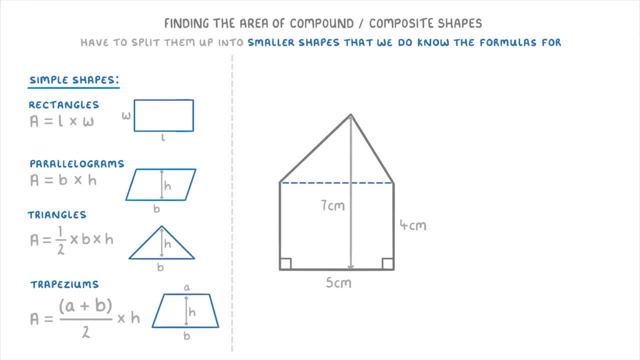 top here, then we can split this shape into a rectangle at the bottom and a triangle at the top. So then all we need to do is find the area of each of them and add the two together. For the area of this rectangle, we need to use this formula in the top left and do length. 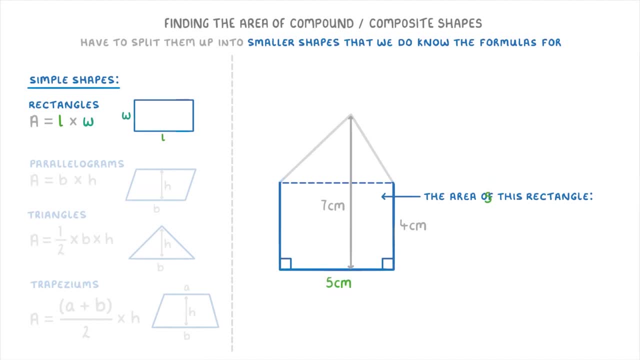 times width, which in our case would be the length of 5cm times the width of 4cm, which gives us 20cm2.. Then to find the area of the triangle at the top we need to use this formula of 1 half times base times height. The base will just be 5cm because it's the same length. 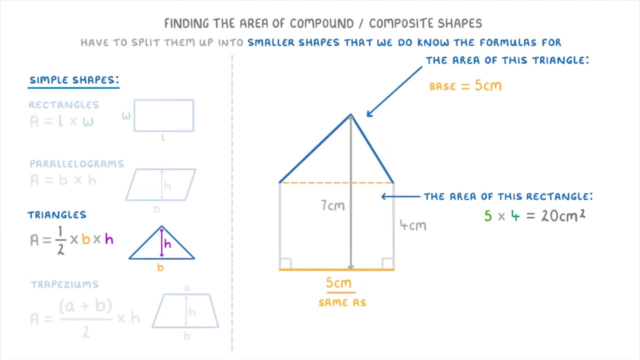 as this base of the original rectangle, So we need to find the area of the triangle at the top. However, we haven't actually been told the height of the triangle, so we're going to have to work that out for ourselves. What we do know is that the height of the 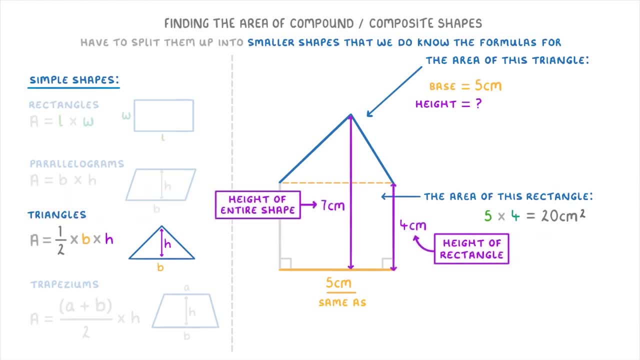 entire shape is 7cm and the rectangle makes up 4cm of that. So the height of the triangle must just be the difference between 4cm and 7cm, which we can find by doing 7 minus 4 to get 3cm. 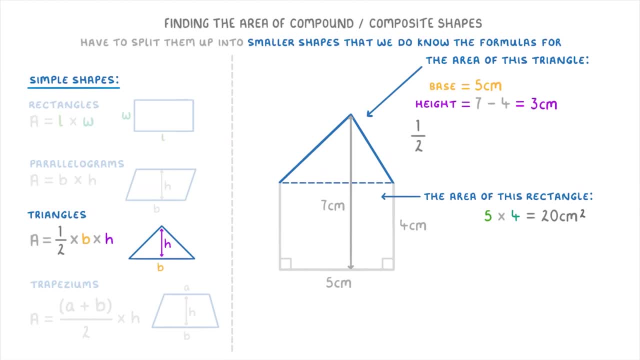 And now that we have our dimensions, we can find the area by just doing 1 half times the base of 5 times the height of 3, and we'll get 7.5cm2.. And then, to finish the question, we work out the total area of the shape by adding together. 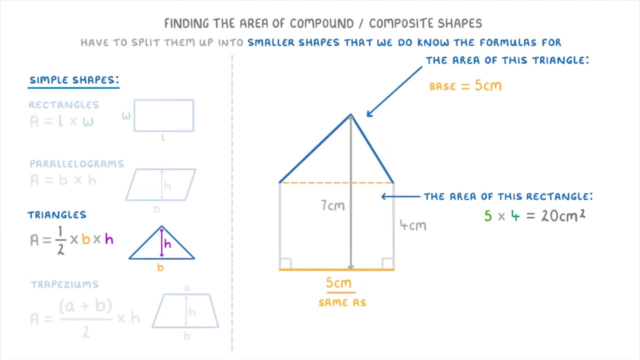 as this base of the original rectangle, So we need to find the area of the triangle at the top. However, we haven't actually been told the height of the triangle, so we're going to have to work that out for ourselves. What we do know is that the height of the 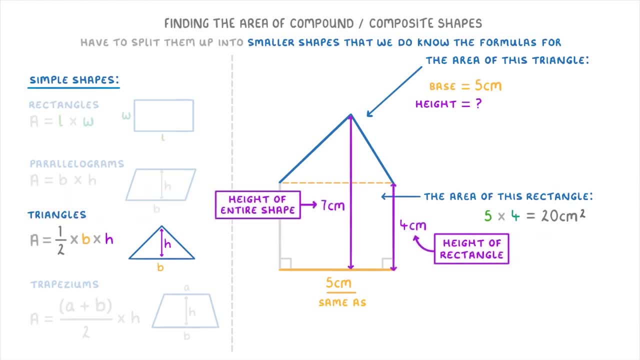 entire shape is 7cm and the rectangle makes up 4cm of that. So the height of the triangle must just be the difference between 4cm and 7cm, which we can find by doing 7 minus 4 to get 3cm. 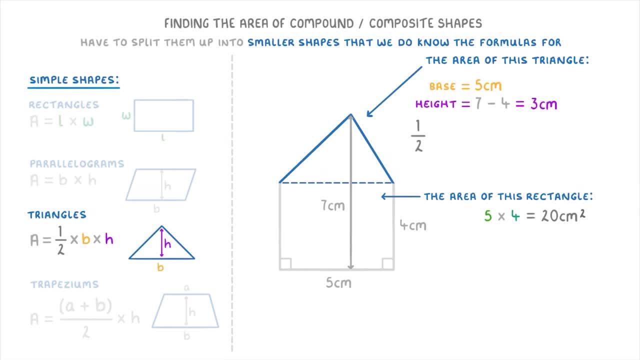 And now that we have our dimensions, we can find the area by just doing 1 half times the base of 5 times the height of 3, and we'll get 7.5cm2.. And then, to finish the question, we work out the total area of the shape by adding together. 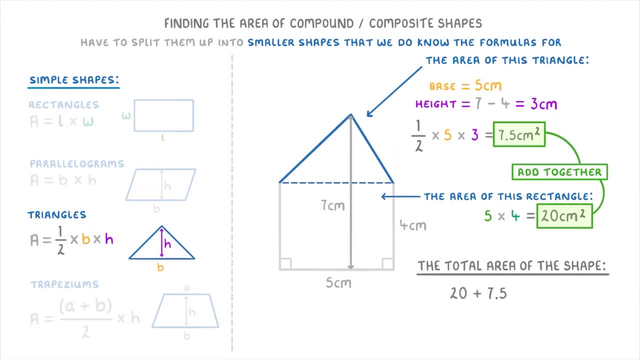 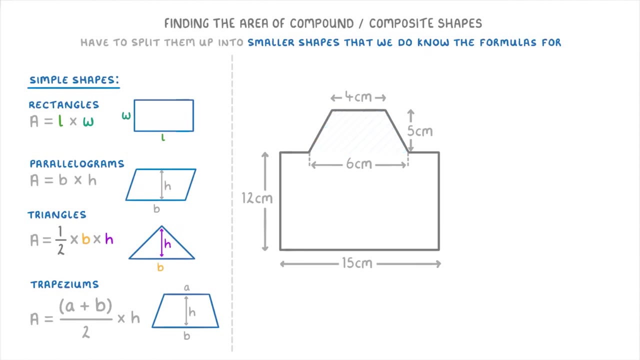 the areas of our rectangle and our triangle. So 20 plus 7.5, which is 27.5cm2.. And that's our answer. If you look at this next one, you can see that this bit at the top is sort of sticking. 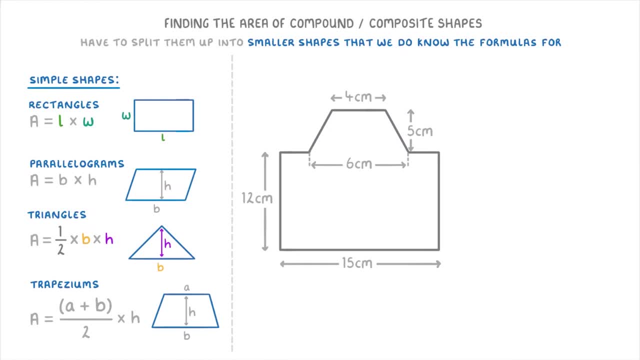 out a bit, And so, to make it easier for ourselves, we can just cut that bit off with a horizontal line along here And we're now left with a big rectangle at the bottom and a small trapezium on top. To find the area of the rectangle we just do length times width again, So 15 times 12,. 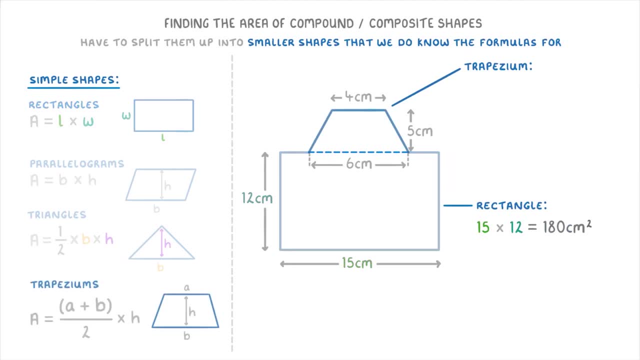 which is 180cm2.. Now let's look at this next one. Let's look at this next one. Next, if you look at the formula for trapeziums in the bottom left, we first have to find the average length by doing a plus b over 2, and then multiply that by the height And 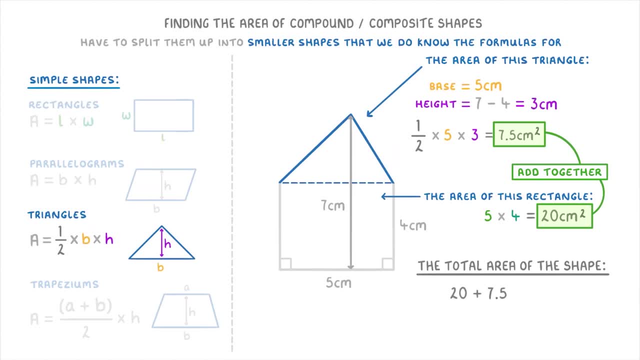 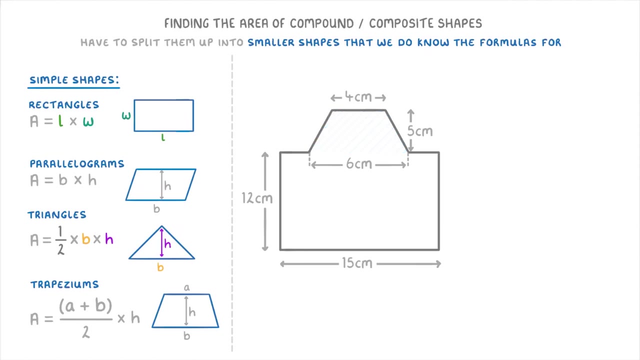 the areas of our rectangle and our triangle. So 20 plus 7.5, which is 27.5cm2.. And that's our answer. If you look at this next one, you can see that this bit at the top is sort of sticking. 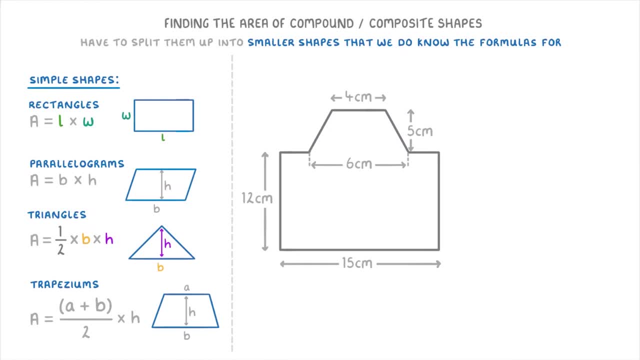 out a bit, And so, to make it easier for ourselves, we can just cut that bit off with a horizontal line along here And we're now left with a big rectangle at the bottom and a small trapezium on top. To find the area of the rectangle we just do length times width again, So 15 times 12,. 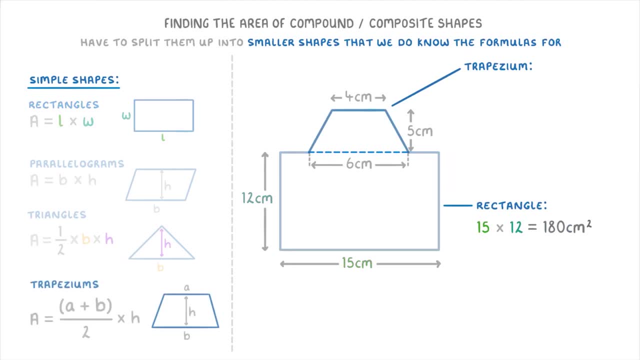 which is 180cm2.. Next up we're going to work out the area of the rectangle. So we're going to do the area of the rectangle and then we're going to work out the area of the rectangle. And next, if you look at the formula for trapeziums in the bottom left, we first have to find: 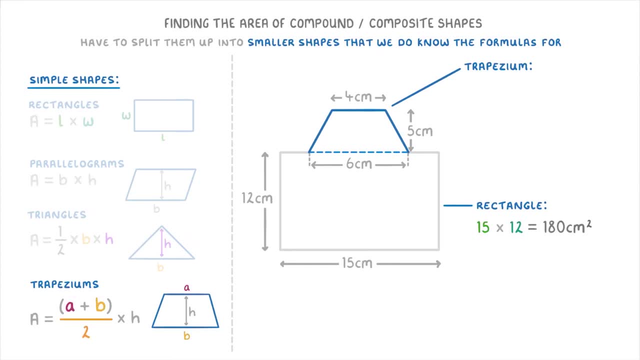 the average length by doing a plus b over 2, and then multiply that by the height. And remember a and b in this formula are just the top and bottom lengths of the trapezium. So in our case we'd do 4 plus 6,, all over 2, and then times that by the height of 5.. 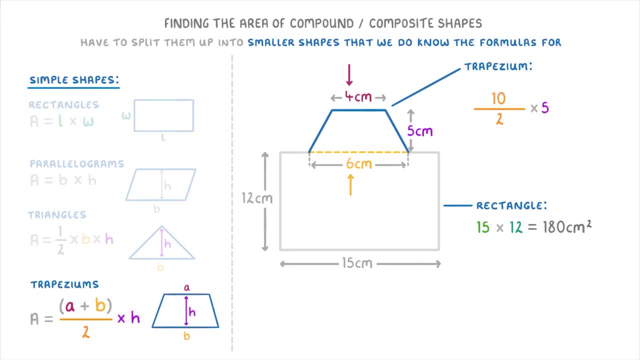 And if we simplify that, the 4 plus 6 is 10, and then the 10 divided by 2 is just 5.. So we have 5 times 5, which is 25cm2.. Then, to finish, we just add together the areas of the rectangle and the trapezium, so 180. 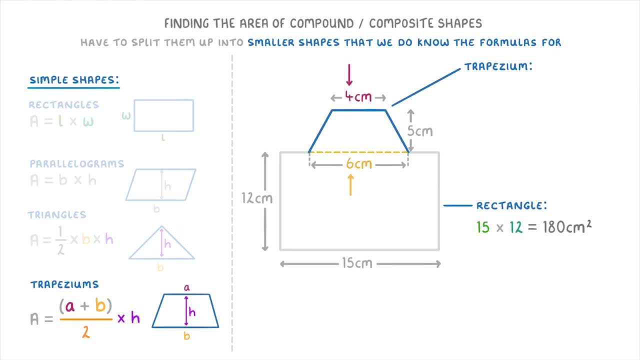 remember, a and b in this formula are just the top and bottom lengths of the trapezium. So in our case we'd do 4 plus 6,, all over 2, and then times that by the height of 5.. 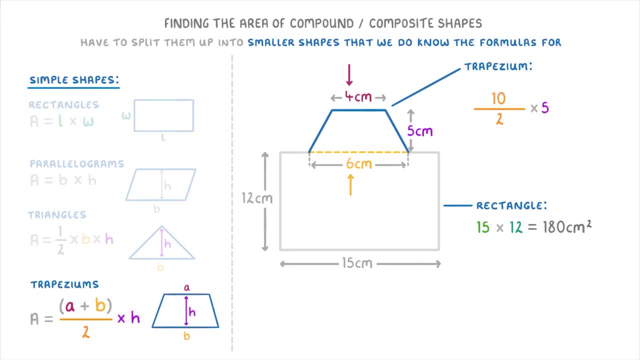 And if we simplify that, the 4 plus 6 is 10, and then the 10 divided by 2 is just 4.5cm2.. So we have 5 times 5, which is 25cm2.. Then, to finish, we just add together the areas of the rectangle and the trapezium, so 180. 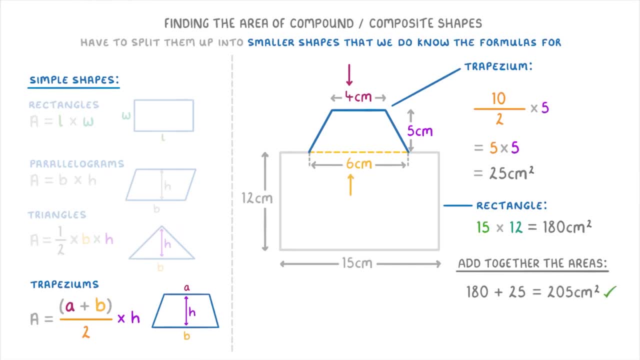 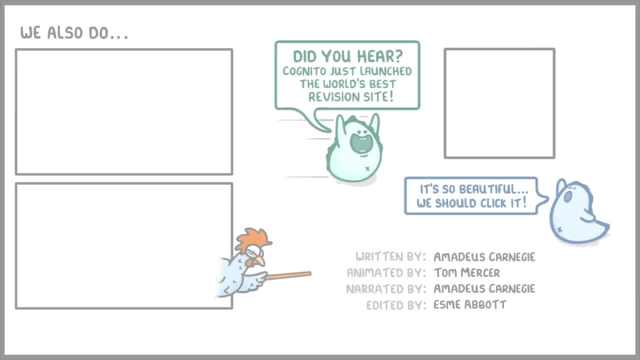 plus 25, to get a total area of 205cm2.. Anyway, that's everything for this video, so I hope it was helpful. If you haven't seen it already, we now have a live past paper website up, so if you're interested in learning, 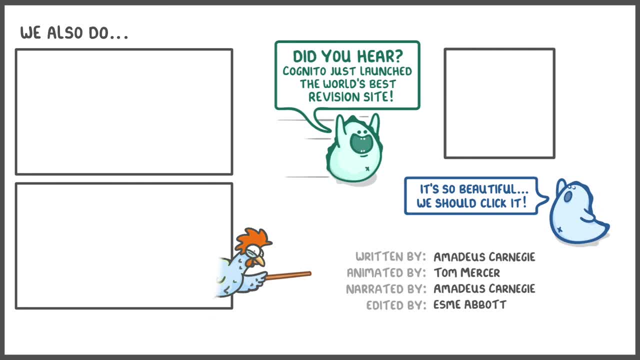 more about trapezium, you can click on the link in the description. So you can just click this button in the top right corner of this screen and you can check out our new website. Hope you enjoy. 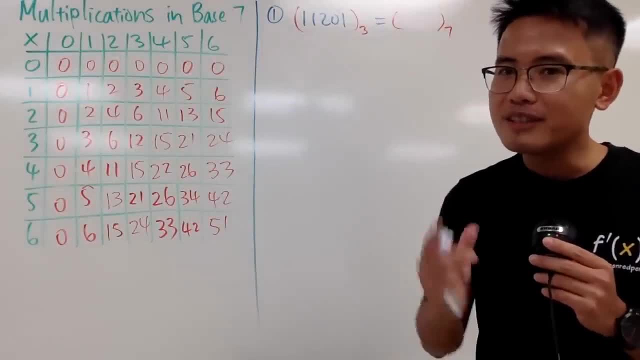 Okay, this is how you convert numbers between two different bases without going to base 10.. We'll do it directly And, depending on what base you want to get to, you should have the times table on the side to help you, Because if not, we will go crazy. 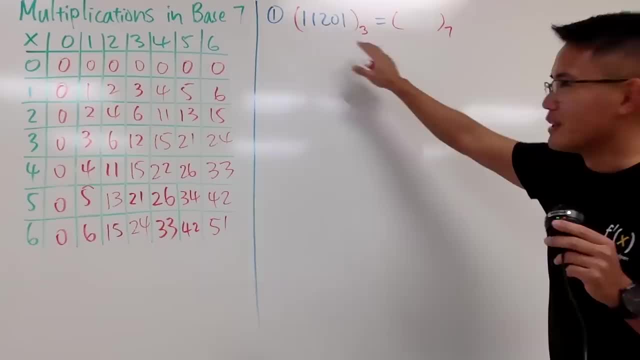 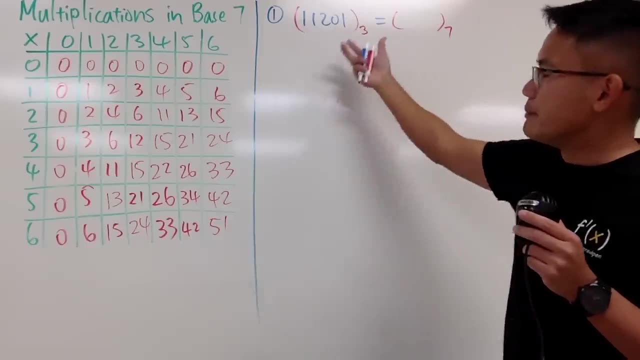 Anyway, I will show you guys how to get to base 7 from different bases, And the first example is 11201 in base 3 to base 7.. So this is an example of how to go from a smaller base to a bigger base. 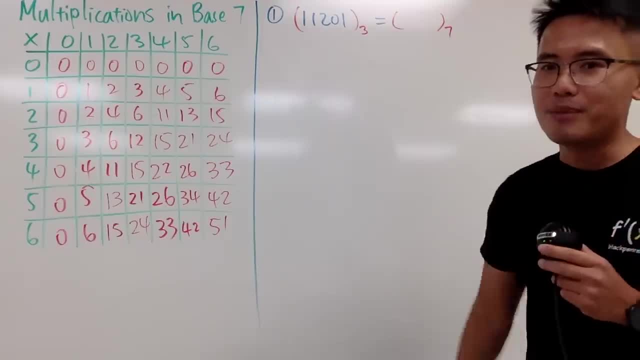 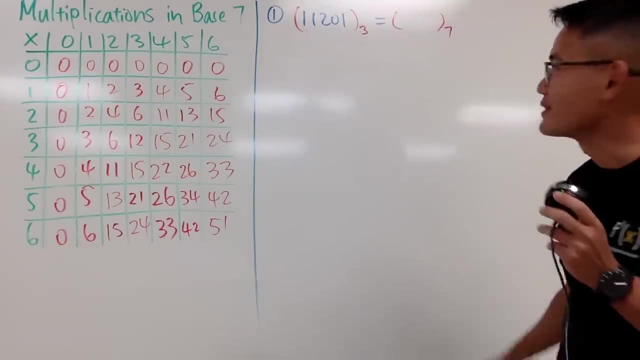 I will show you guys another example to go from a bigger base to a smaller base. And here is the times table in base 7.. In fact I have a video on this. If you haven't seen it, be sure you guys go check that out. 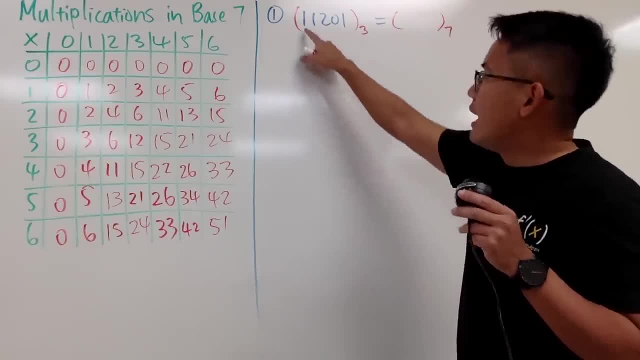 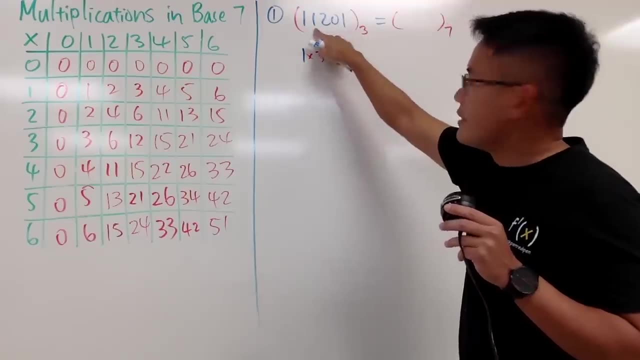 Okay, here we are going to start by expanding this, And we'll do it this way, Starting from the number from the left right. here we have 1., And then we multiply by 3. And then I add the next number, which is 1.. 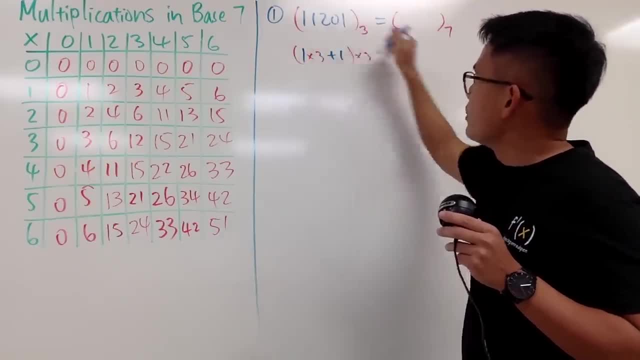 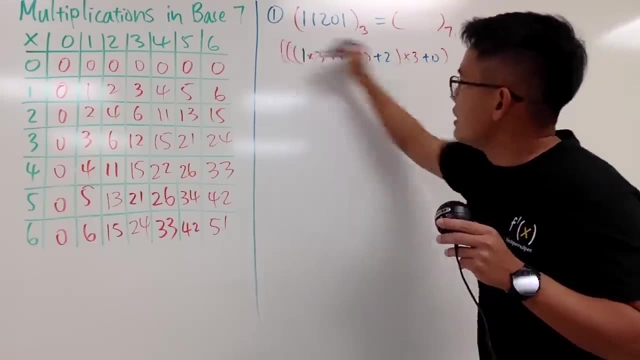 And then we multiply by 3. And then we continue, We add 2. And then we put parentheses, And then we multiply by 3. And then we add 0. Put parentheses And then we multiply by 3. And then we are going to add the 1 right here.